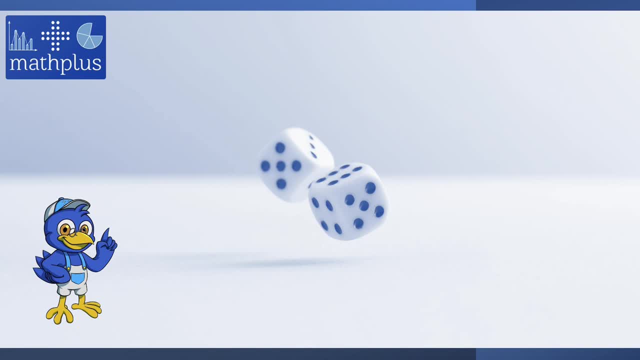 the results of each trial performed. We don't know what their outcomes will be. That's what makes them uncertain. We are not 100% sure about the outcomes, But we can use mathematics to describe the likelihood of the outcomes of the experiments. We can use what we call the 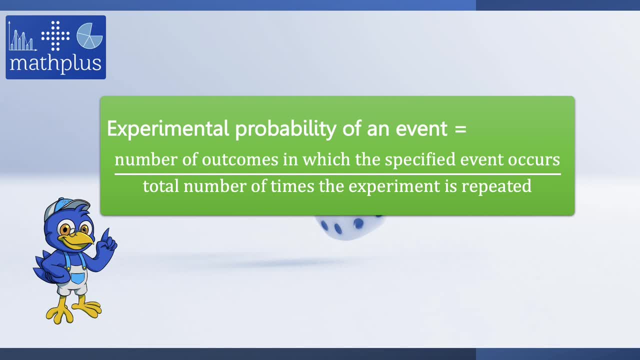 experimental probability of an event. So this experimental probability can allow us to understand the likelihood of outcomes By first repeating the experiment many, many times. When we repeat the experiment many times, we can compute the experimental probability of an event using the formula shown in the screen. 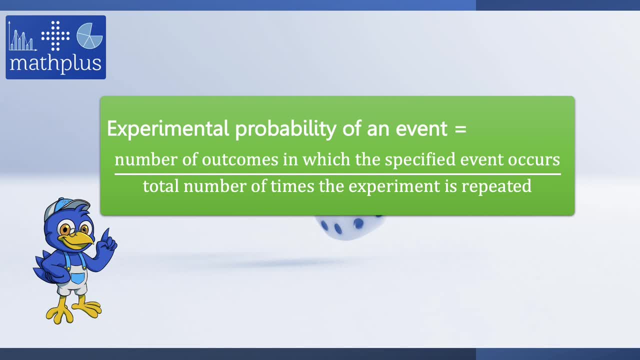 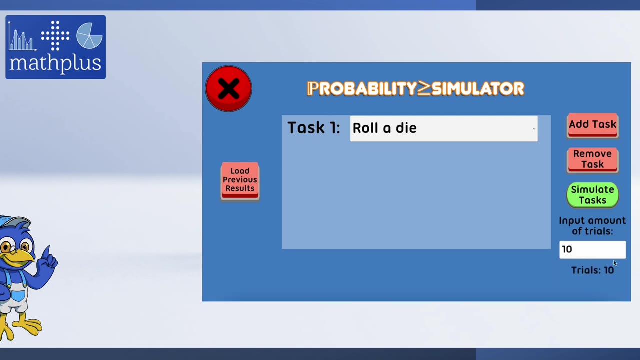 We first count the number of outcomes in which the specified event occurs And we divide this number by the total number of times that the experiment is repeated. Now let's try an example. Let's just focus on rolling a die and let's do 10. 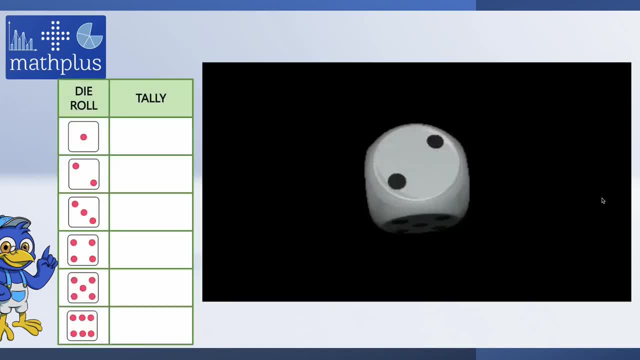 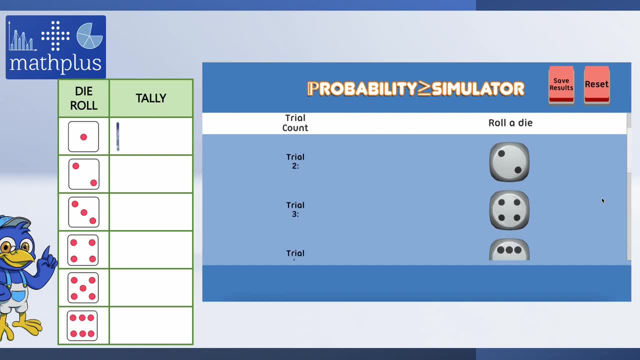 trials. We will record our outcomes in this table. So, as we can see, trial number one, the outcome is one. For trial number two, it's two. For trial three, it's four. For trial four, it's six. For trial five, it's four. again For trial six, it's one, followed by another one For trial eight, 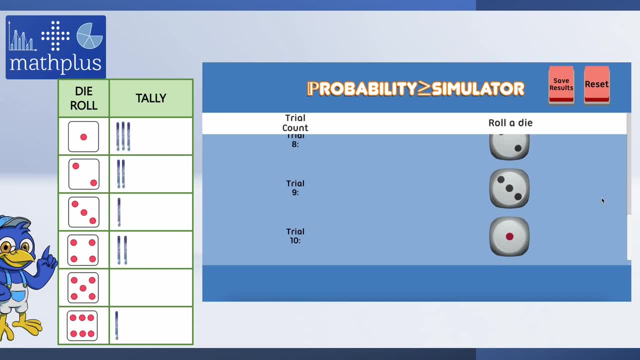 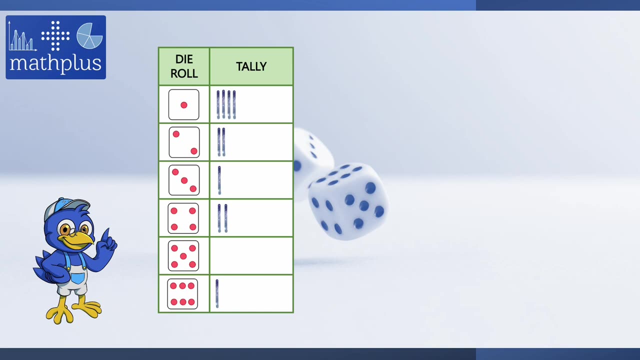 2,, trial 9, the result is 3, and finally, in trial 10, the result is 1.. We can now use this table to compute the experimental probability for each outcome. For example, since we got the result 1 four times out of the 10, 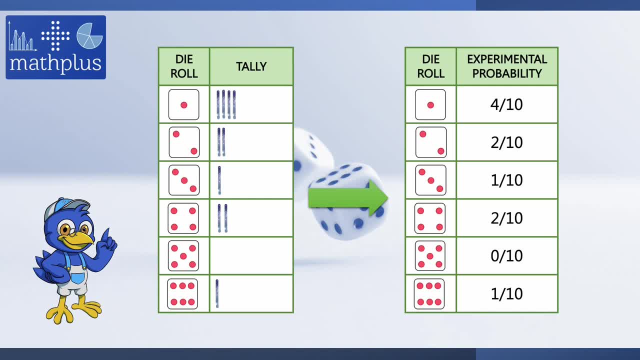 trials, its experimental probability is 4 over 10.. Similarly, we got 2 two times in the 10 trials, so the experimental probability for 2 is 2 over 10.. And another example: we didn't get any outcome 5 during our 10 trials, so the 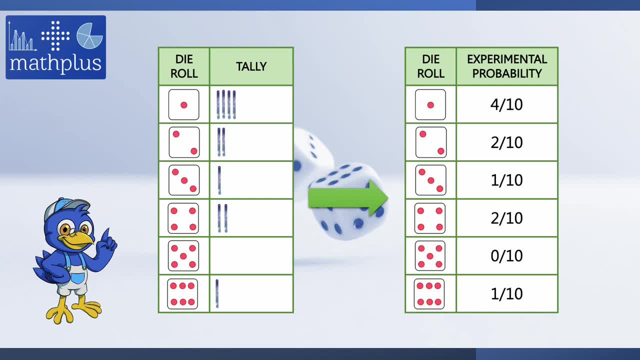 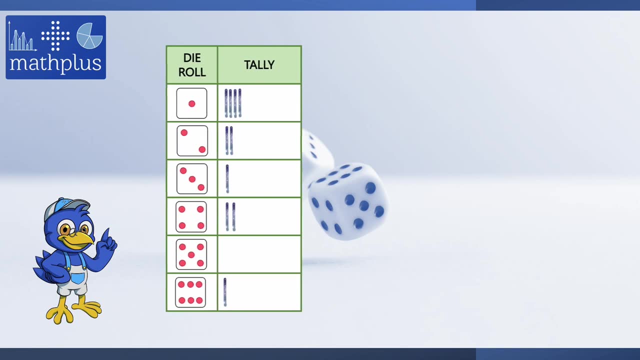 experimental probability for 5 is 0 over 10.. Now take note that we only perform a few trials. it's only 10, so our experimental probability might not be very accurate yet. Oh, it seems Banoy also has some questions for us. Okay, Banoy's. 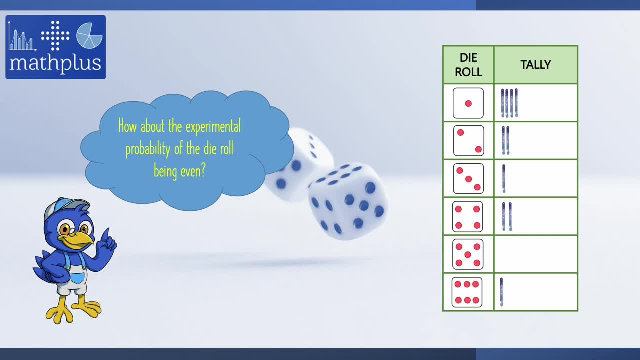 question for us is: how about the experimental probability of the diorol being even? Well, among the six possible outcomes, we have 2,, 4, and 6 as even outcomes And, as we can see in the table, there are 5 outcomes in which 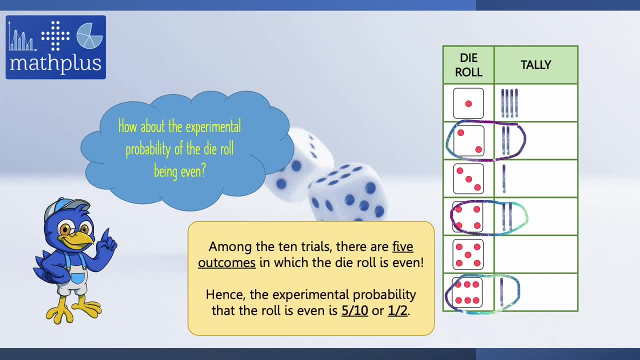 the diorol is even. So the experimental probability that the diorol is even is equal to 5 over 10 or 1 half. Okay, it looks like Banoy has one more question. How about the experimental probability of the diorol being less? 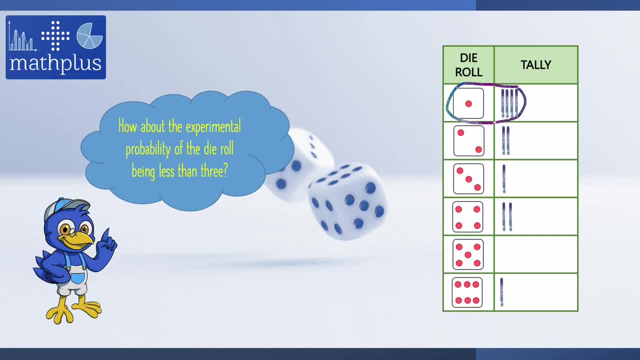 than 3?? Okay, the diorols that are less than 3 and 2.. We can see that there are 6 outcomes in which the die roll is less than 3.. Therefore, the experimental probability that the die roll is less than 3 is 6 over 10 or 3 over 5.. 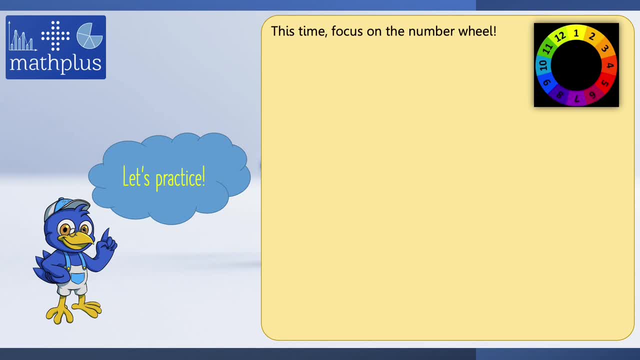 Okay, you should practice This time. focus on the number wheel Using your MathPlus probability app. spin the number wheel 15 times and record the outcomes in a table. Then compute the experimental probability of each possible outcome. Also compute the. 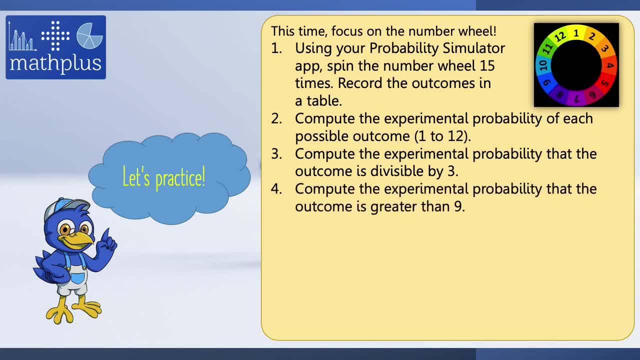 experimental probability that the outcome is divisible by 3, that the outcome is greater than 9.. In step 5, you have to repeat steps 1 and 2, but this time you have to spin the wheel 25 times And again repeat steps 1 and 2,, but this time spin the wheel 35 times. Based on steps 5 and 6,. 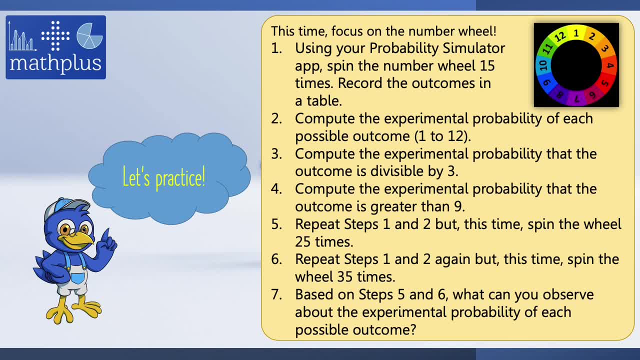 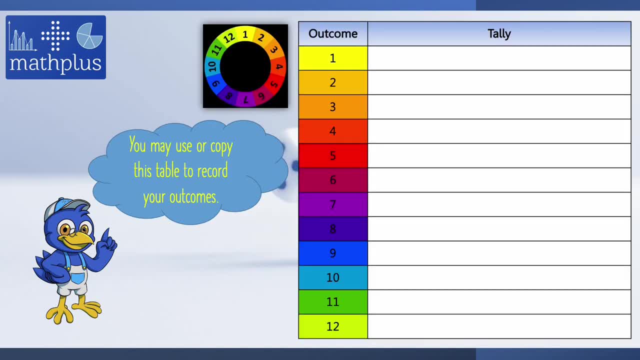 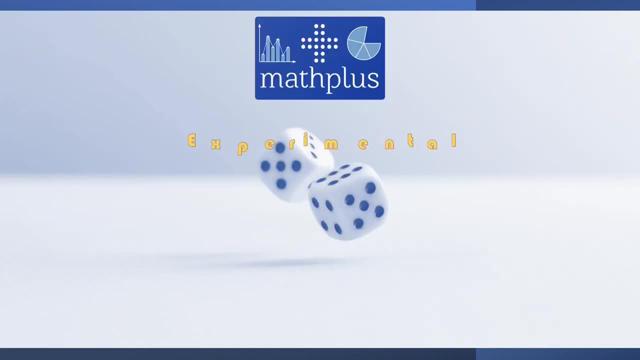 what can you observe about the experimental probability of each possible outcome? So that's your practice. Oh, Banoy has something for you. You may use or copy this table to record your outcomes. Thank you, Banoy. Well, that's the end of our activity for today. Banoy say goodbye.